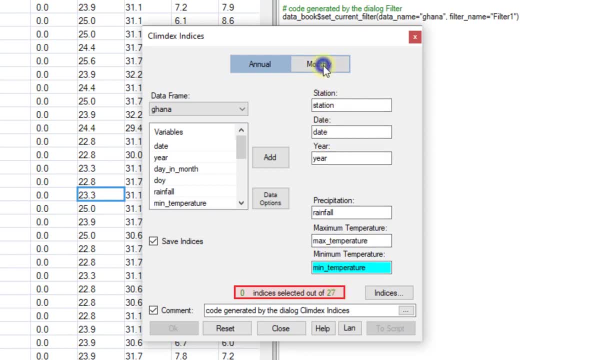 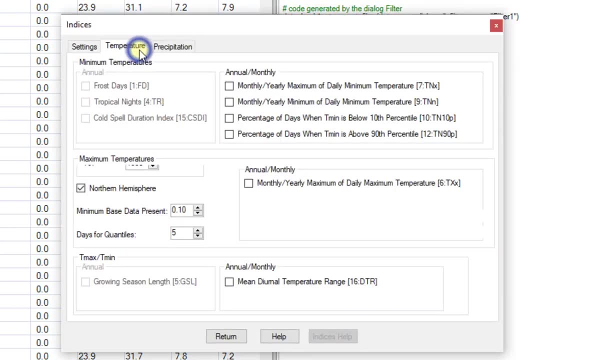 There are 27 indices, of which 11 are also available monthly, which we need here. Clicking on the indices button, choose the temperature tab. Select the five elements shown. They are the extremes for TMax and TMin, together with the mean diurnal range. 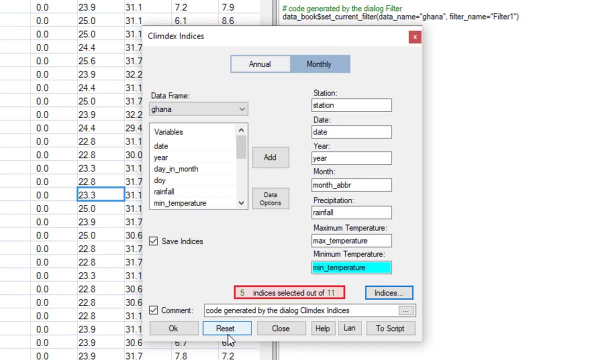 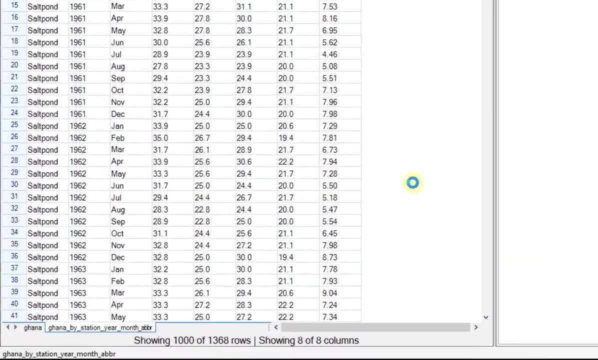 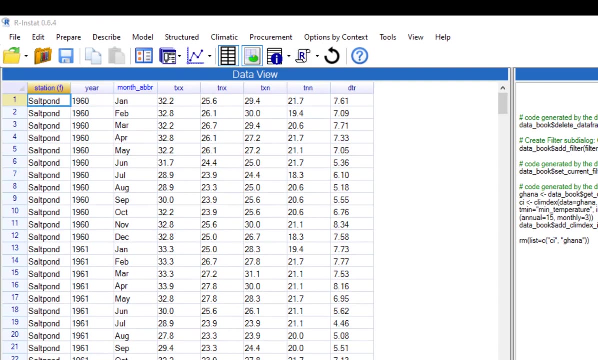 The main dialogue confirms that five have been selected. Press OK. Are the results the shape that we would expect? There are eight variables, namely the station, year and month, followed by the five summaries that we chose. There are 1368 rows of data. 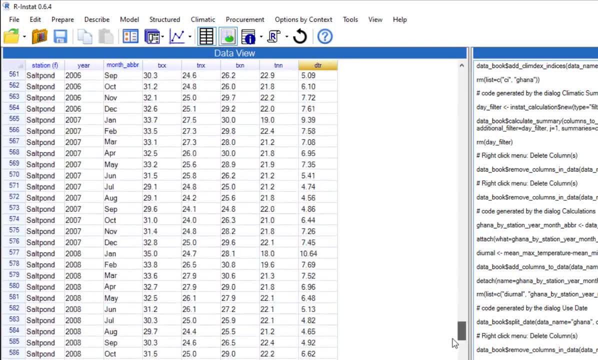 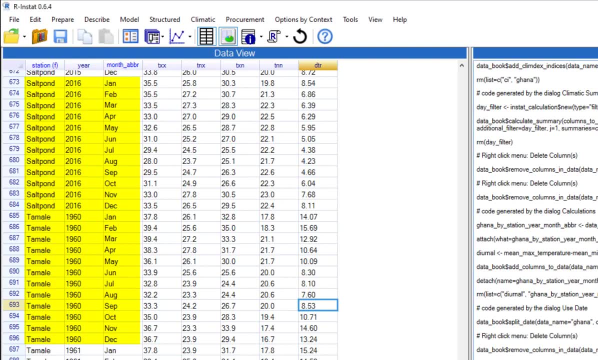 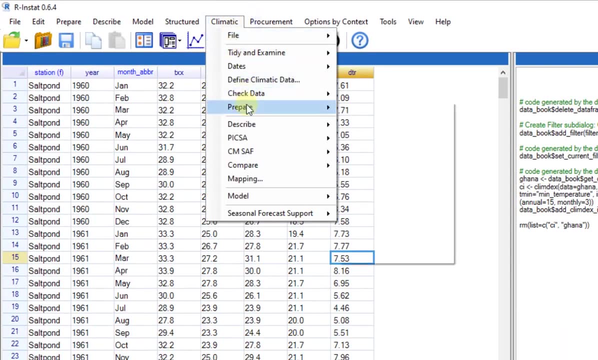 That's two stations by 12 months of the year, from 1960 to 2016.. So 57 years 24 times 50 is 1200, so that seems about right. Now use the climatic summaries dialogue to see how the results compare. 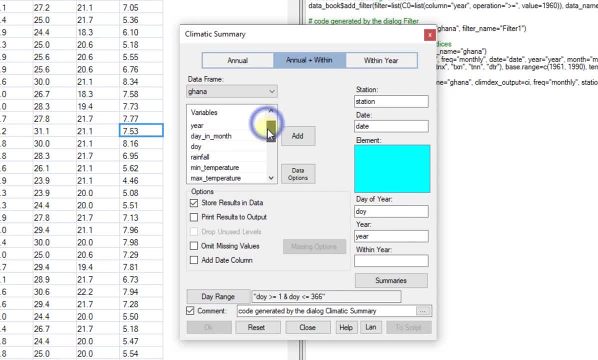 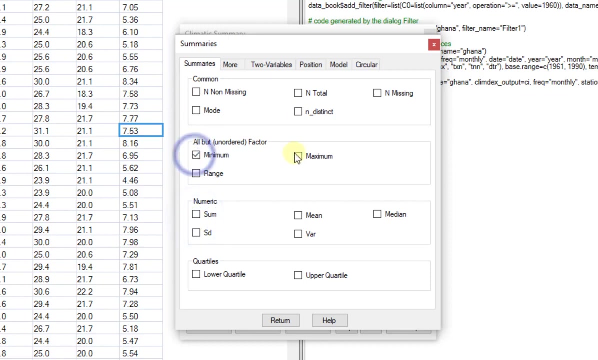 Choose annual and within We include the two temperature variables as shown and we use the month as the factor. The missing values checkbox remains unticked. as we're being cautious From the summaries, choose to include just the extremes and the mean Return, then OK. 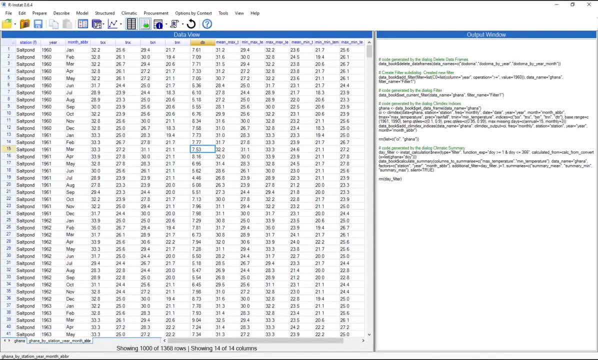 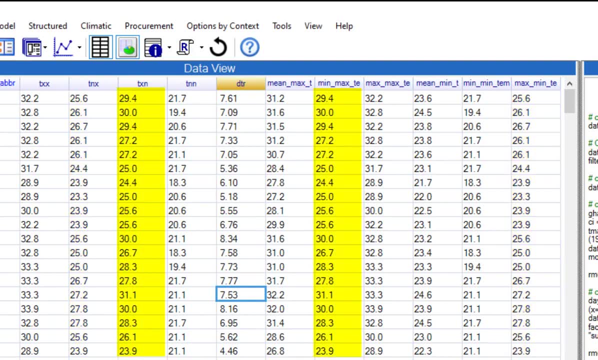 This adds six new variables into our monthly data frame. Four of the summaries should be the same as we found from Climdex. Let's check. Well, that's a relief. Now that we've seen that they are the same, we can delete the second occurrences. 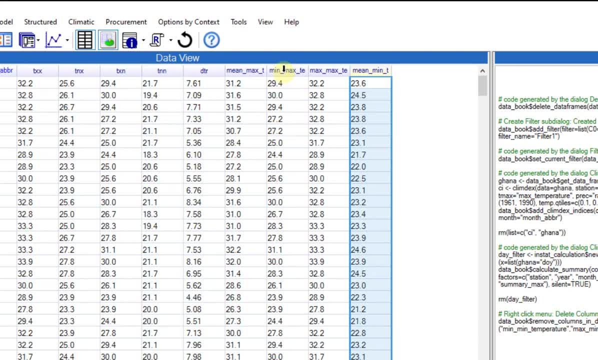 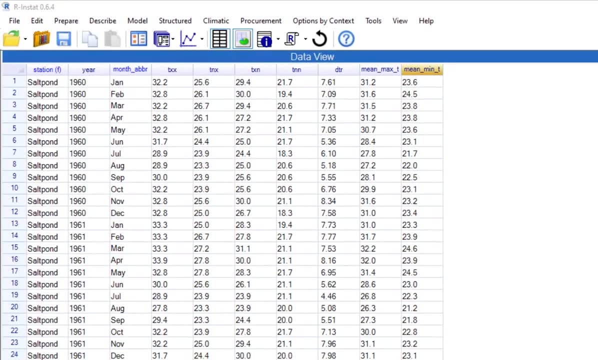 They're not needed twice. There are now seven summary variables. In particular, the monthly means are added to the temperature extremes from Climdex. We can understand why the means are not available from Climdex, Because it's a system designed to study extremes. 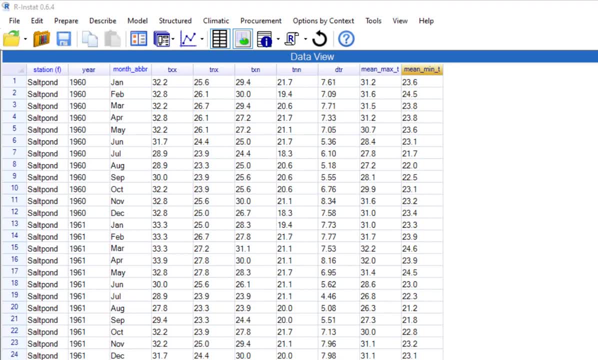 Their emission is not a problem as long as users don't limit their analyses to only the indices in Climdex. If studying trends, we can see that the indexes in Climdex are not limited to only the indices in Climdex. If studying trends in temperatures, it's important to consider the extremes. 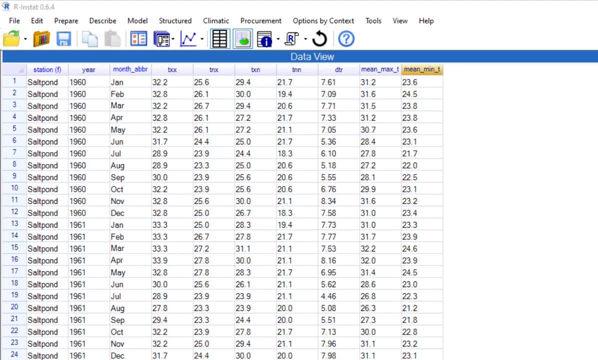 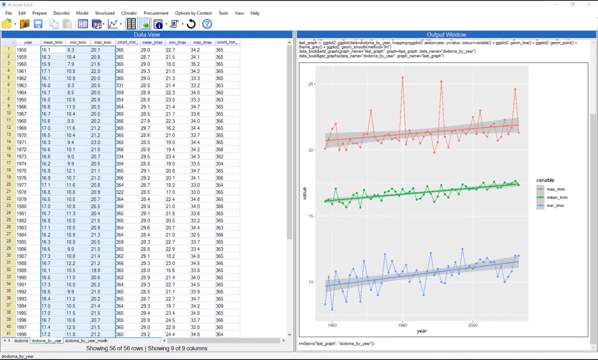 But if their trend isn't different, then the overall trend is estimated more precisely from the mean. The mean is calculated from all the days in each month, while the extremes are just from a single day. This point is clearer with annual summaries, as was shown in the tutorial. 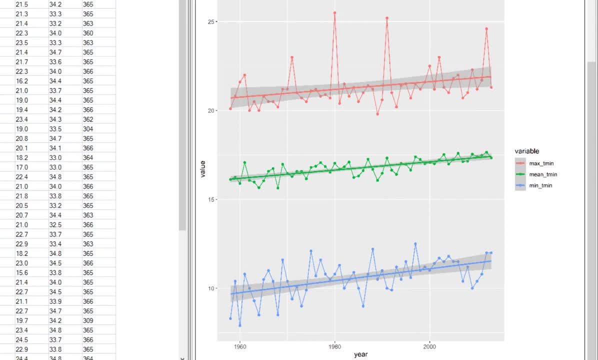 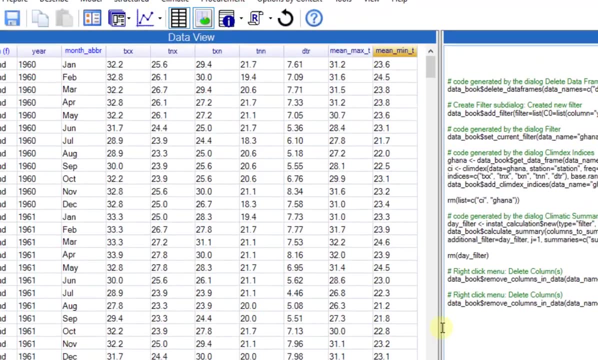 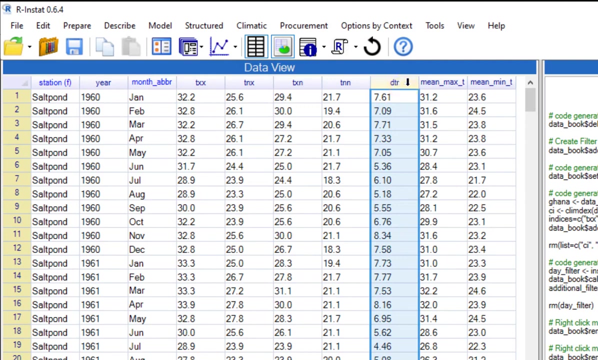 Going back to the Dodoma data, the shaded areas are much narrower for the mean line than for the extremes, In contrast. the seventh summary is the mean diurnal range. This is from Climdex and is not available from the climatic summaries dialogue. 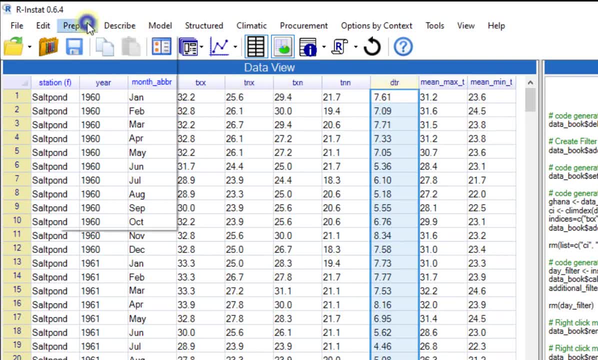 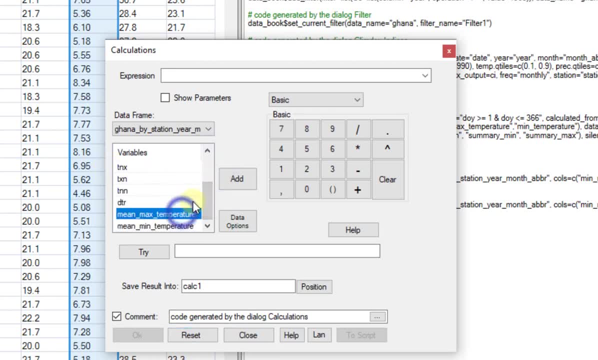 Is it just the difference between the means of Tmax and Tmin? Let's check using the calculator. Let's check using the calculator There. simply take the mean of Tmax and subtract the mean of Tmin. Check with the trie. It works and seems to be giving the same answer for the first years too. 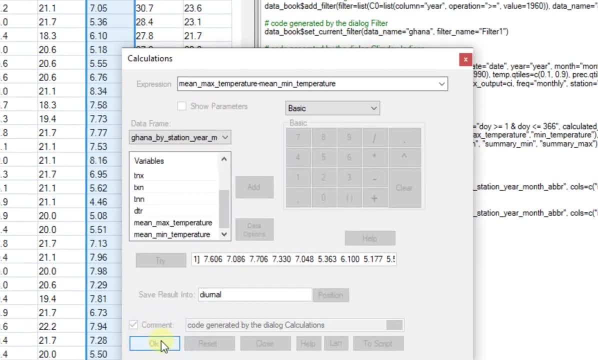 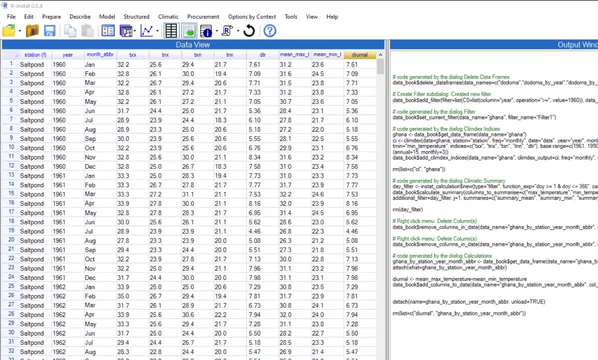 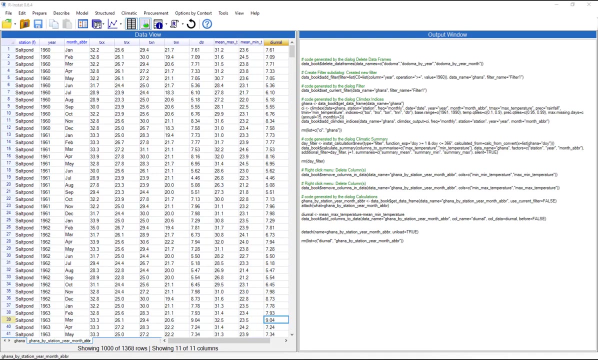 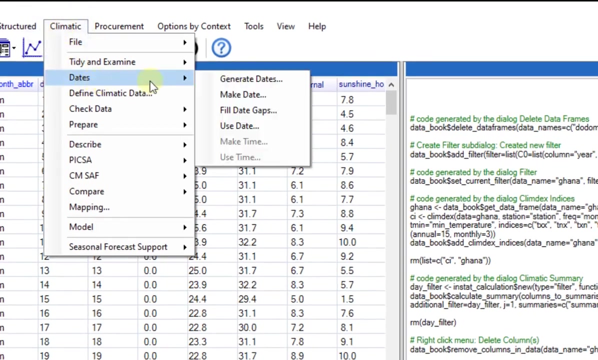 Call it diurnal. Good, they are the same, so we did understand it correctly. Finally, we will respond to a request for the temperature extremes and means on a 10-day basis. This is easily done. Return to the daily data and use the date dialogue. 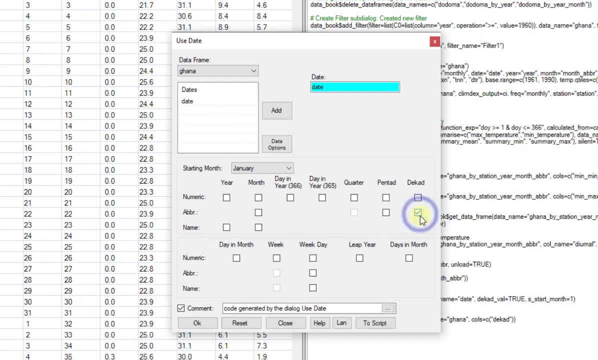 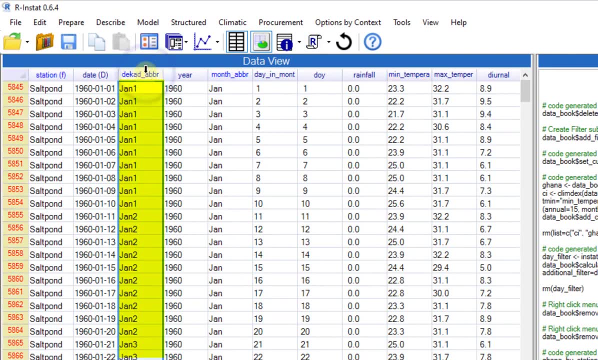 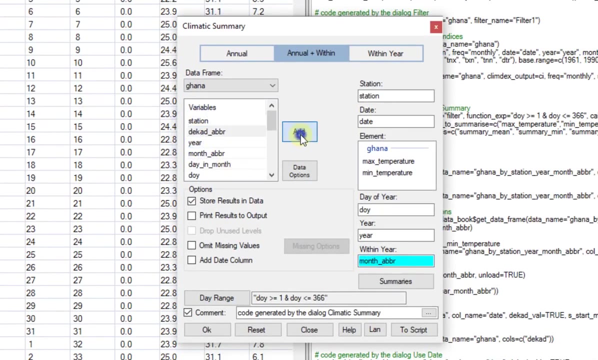 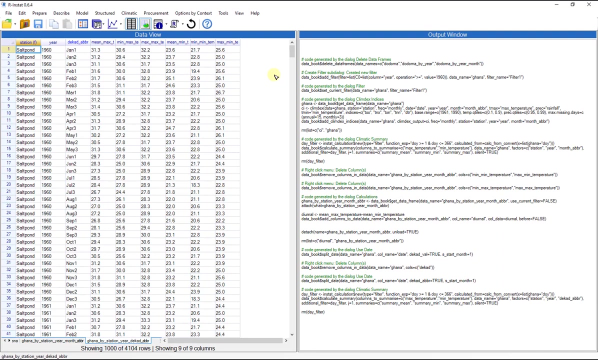 Select the DCAD option and press OK. This adds a DCAD variable to the data. Now we go back to the climatic summaries. Here we make our DCAD variable the within factor. So there you have it, Starting from the daily data. the first stage of analysis is a summary. 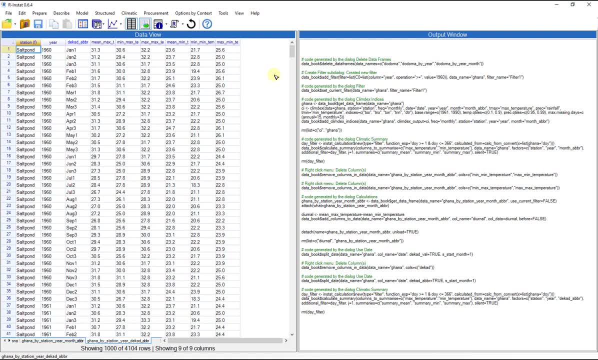 For temperatures, the mean is obvious, but there are many others, including the extremes. You may require a standard summary, perhaps through Climdex, Or you may want flexibility to respond to specific questions. Or you may want flexibility to respond to specific questions. 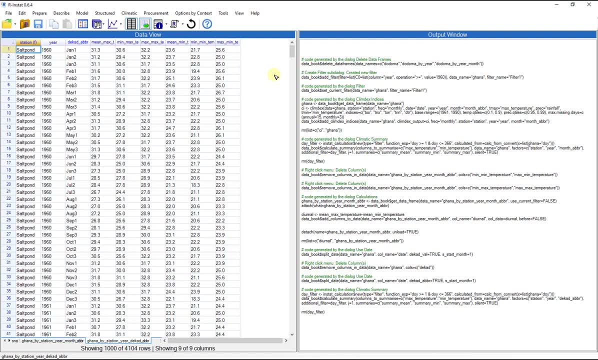 As we showed as well, And the summary may be annual, Or it can include a seasonal component, like quarters, months or decades. Then the second stage is to process these summaries. Let's finish with a graph, A line plot, just as you saw earlier in this video. 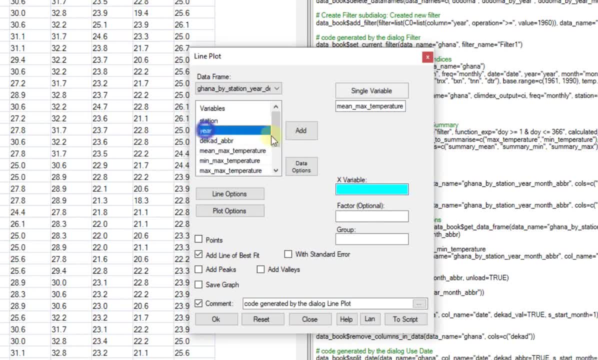 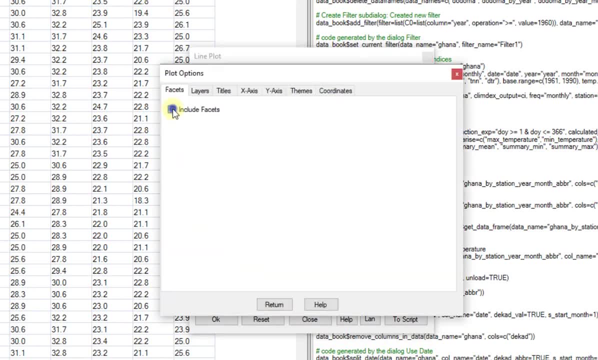 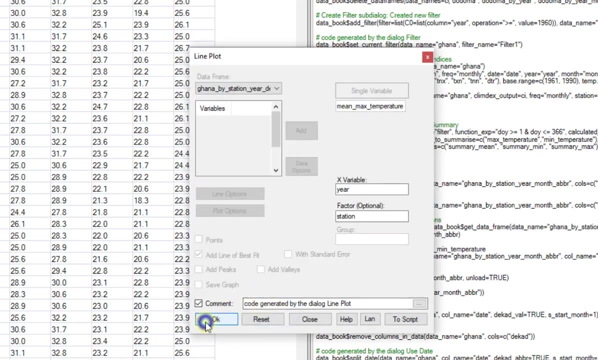 We use mean Tmax by the year for each station. We have a line plot, We have a line of best fit And we go to plot options to include facets. Use the DCAD as the facet. Well, that seems good value: 36 graphs for the price of 1.. 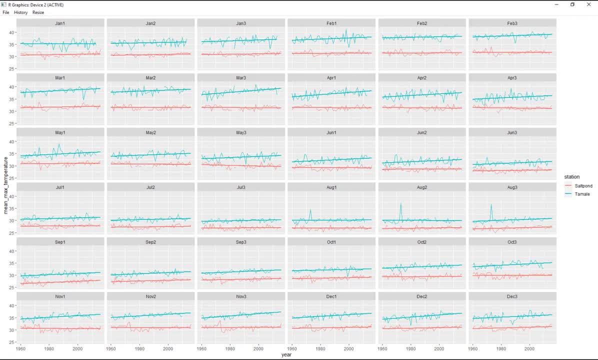 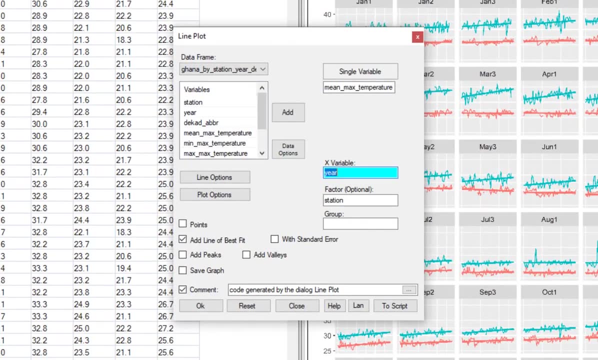 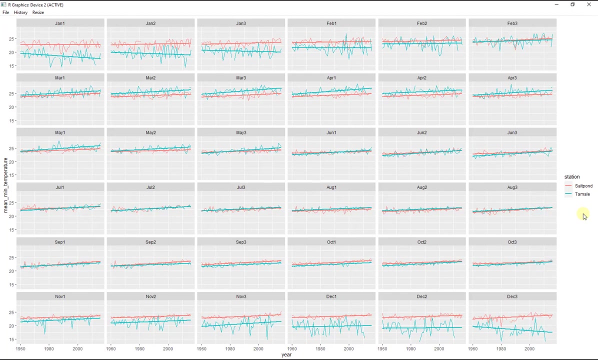 Or maybe it's confusing. Is the pattern the same for Tmin? Return to the dialog And change the element, And change the element. Well, that's at least interestingly different For Tmin. the lines seem almost identical for the whole summer.